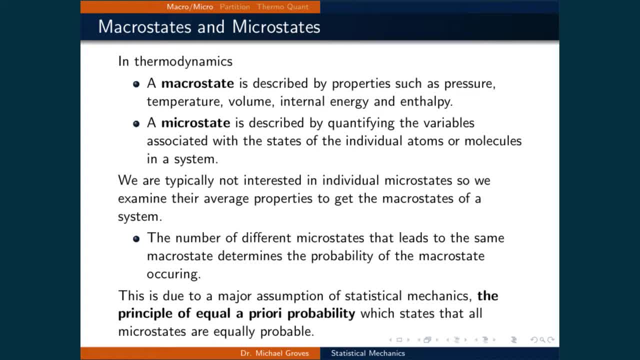 similar microstates. We are generally not interested in individual microstates, since it's the macrostate of a system that we measure as a property of the system. One major assumption in statistical mechanics is the principle of equal a priori probability, which states that all microstates are equally probable. This means that the number of different microstates 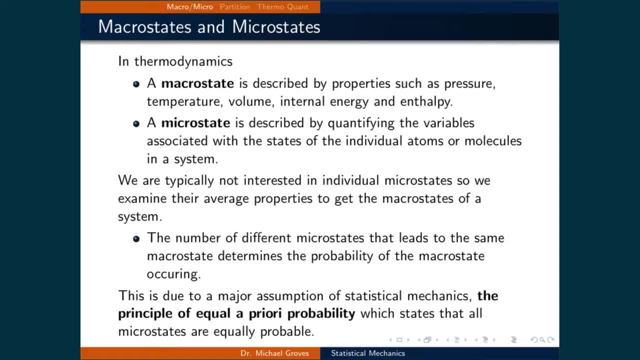 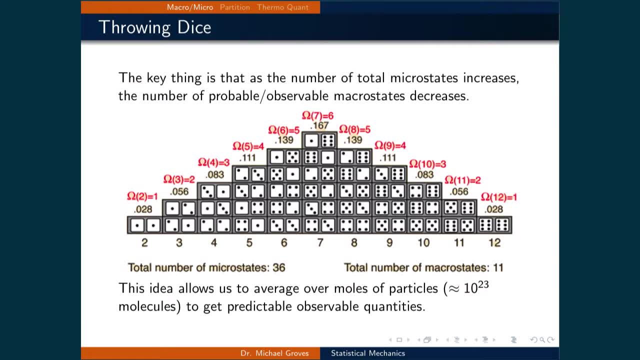 that is a member of the same macrostate determines the probability of the macrostate to be equal. If the number of microstates is equal, the probability of the macrostate to be equal to the number of other microstates is equal to the probability of the macrostate to be. 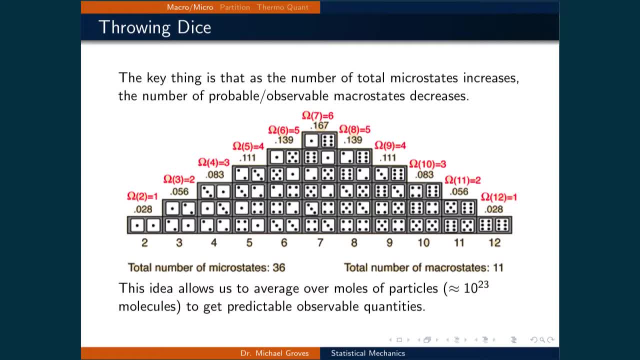 equal. So let's look at an example of a macrostate occurring. These points can be easily seen with an intuitive example throwing two dice. The image shows all possible face value combinations of two dice ranged according to their total. A microstate in this case is the face value. 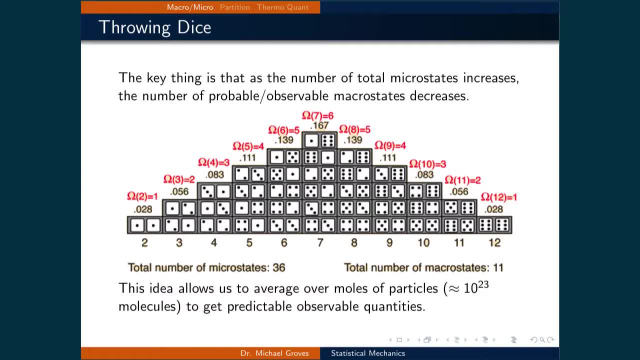 of the two dice. So a microstate would be when one dice reads one and the other also reads one. A macrostate in this case is the total from both dice. Since each microstate is equally likely, then the number of microstates in a macrostate determines how likely a given. 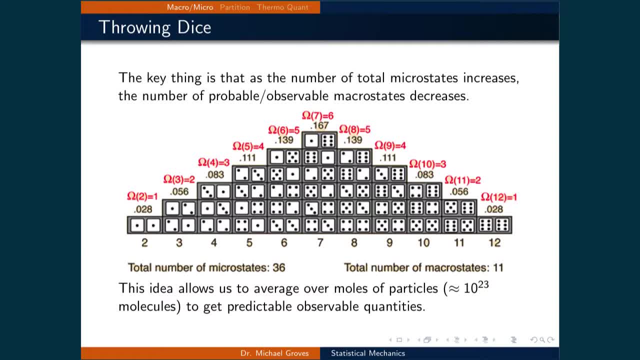 macrostate is, As can be seen in the image. 7 is the most probable macrostate, since there are six combinations of microstates that give 7.. 2 and 12 are the least likely macrostates, since there is only one microstate for each. There are a total of 36 microstates and 11. 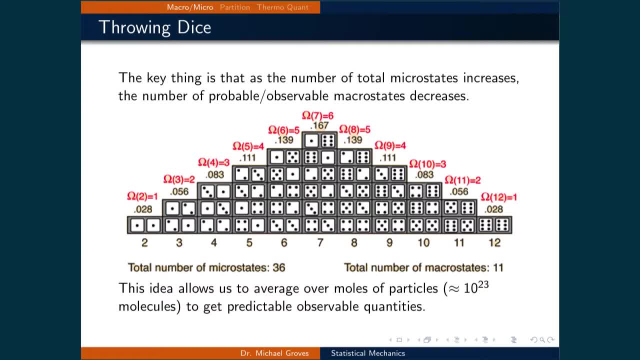 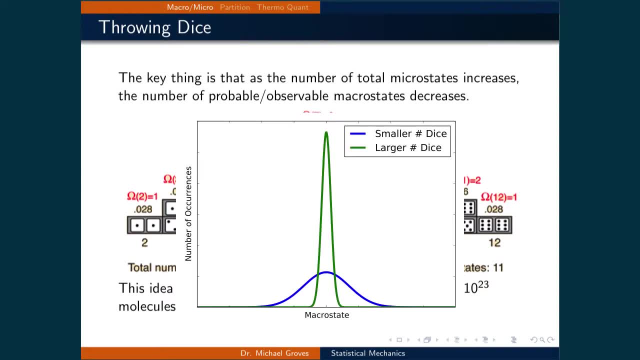 macrostates for this system. An important observation here is that the number of microstates in a macrostate determines how likely a given macrostate is. As the number of total microstates increases, the number of probable or observable macrostates decreases- In the dice example, increasing. 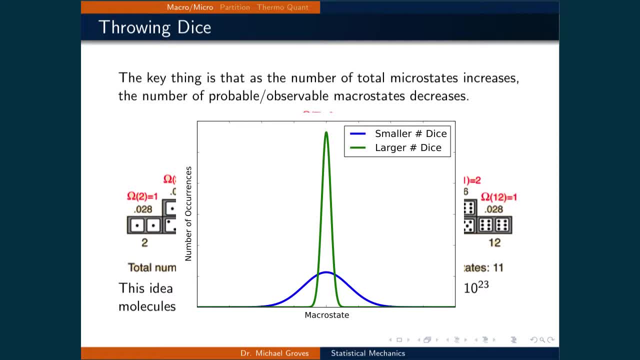 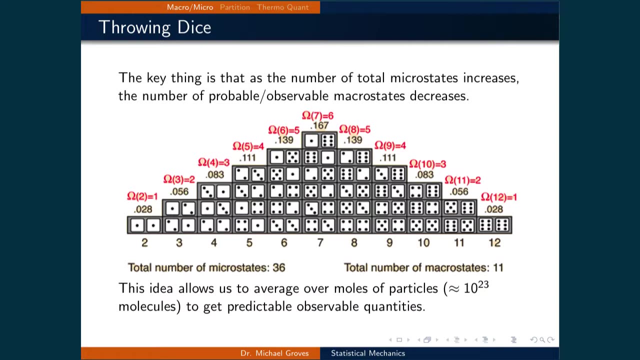 the number of microstates means throwing more dice. If we were to throw more dice, say 10 or 100, the broad distribution seen with the two dice becomes much thinner. The most likely macrostate becomes very probable relative to all others. This phenomenon is what allows us to average over moles of particles and get predictable. 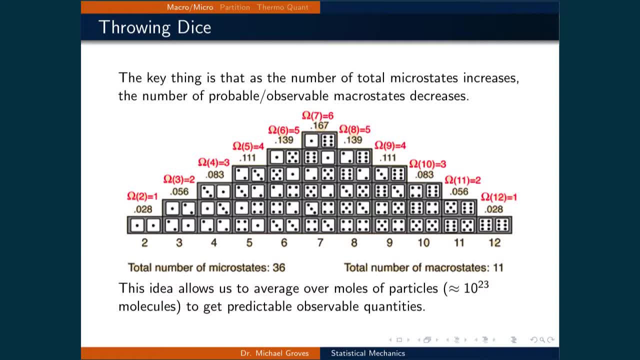 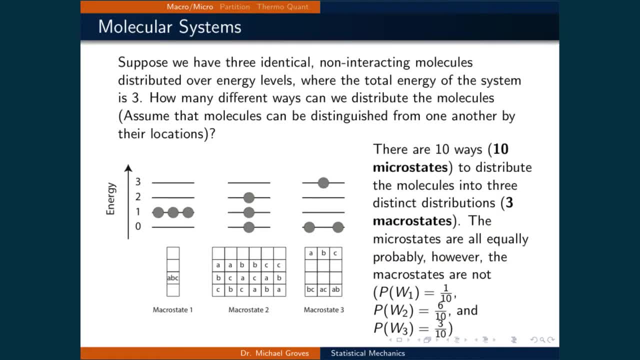 observable quantities, since they tend to be the only probable ones. Consider a second example. Suppose we have three identical non-interacting molecules distributed over energy levels where the total energy of the system is equal to 3. How many different ways can we distribute the molecules? Assume that the molecules can be distinguished. 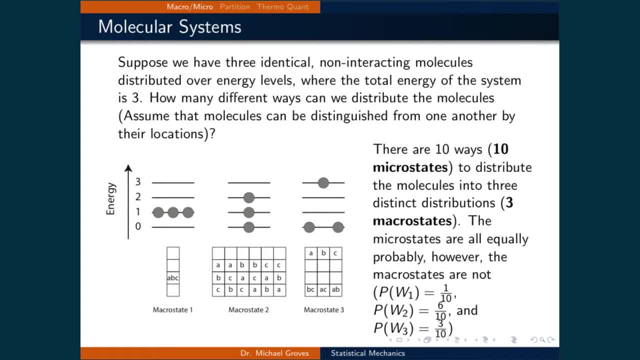 from one another by their locations. The illustration on the left shows that there are, in general, three ways to distribute the molecules in the energy levels. These are the macrostates. For each macrostate there are a different number of microstates. For macrostate 1, there is only one way to put all three molecules into energy level. 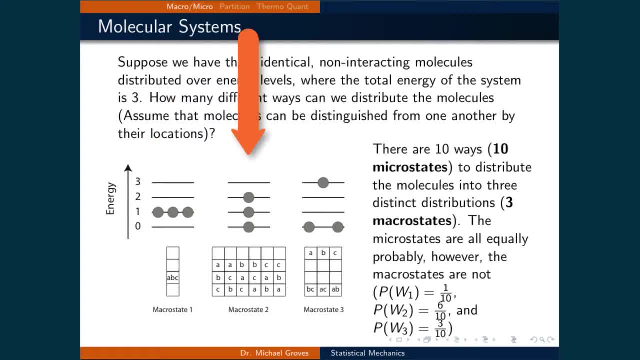 1. For macrostate 2,, there are six ways to arrange the three molecules on their own, in energy levels 0,, 1, and 2.. Finally, there are three ways to distribute the three molecules where one is in energy level 3 and the other two are in energy level 0. 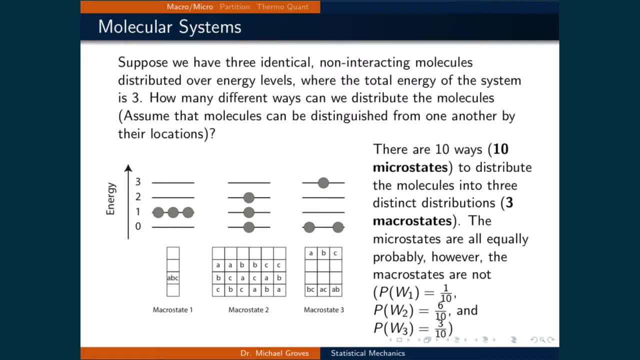 Let's look at another example. Since there are ten ways to arrange the molecules so that the total energy is 3,, then that means the most probable macrostate is number 2.. The general formula for calculating the number of microstates in a distribution, w, is equal. 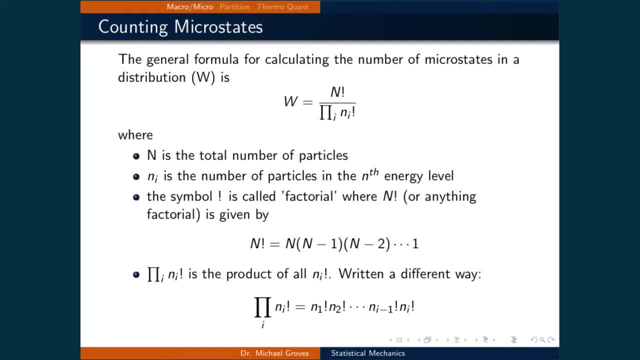 to n factorial divided by the product of ni factorial. And this is where n is the total number of particles, ni is the number of particles in the nth energy level. The exclamation mark is called factorial where n factorial or anything factorial is given by n times n minus 1, times n minus 2, all the way down. 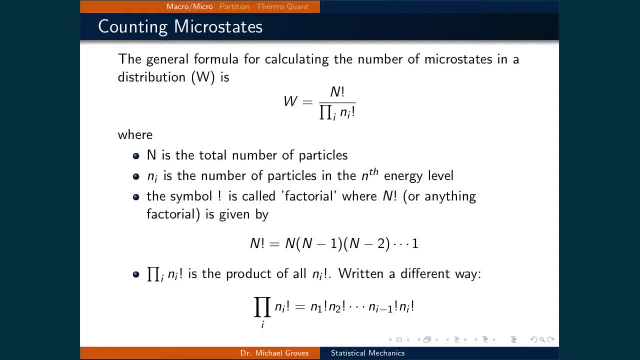 until it's times 1.. As a side note, 0 factorial is also equal to 1.. The large pi symbol means the product of all that follows. In this case it is referring to the product of all ni factorial Written in a different way. it would be written as: 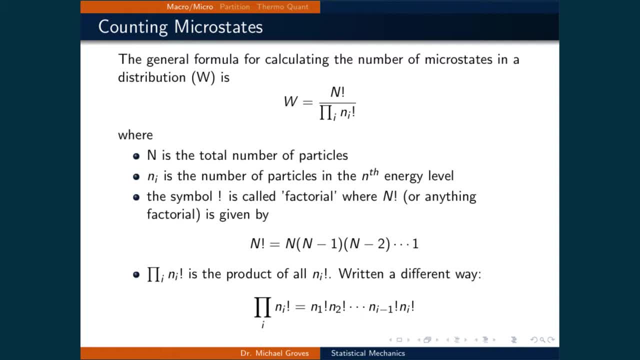 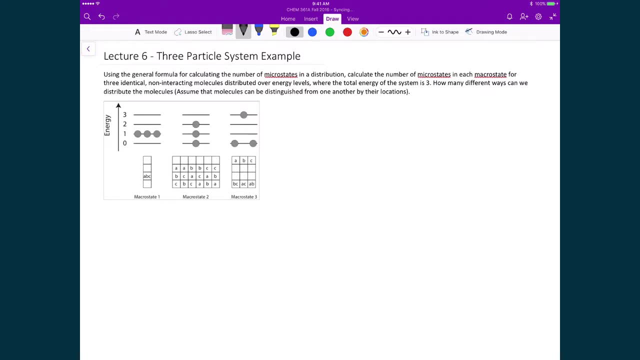 n1 factorial times n2 factorial, all the way to ni minus 1 factorial, ni factorial. Let's use this now in practice to determine the number of microstates in a distribution, using the exact same problem that we had already analyzed with our three-particle system, where 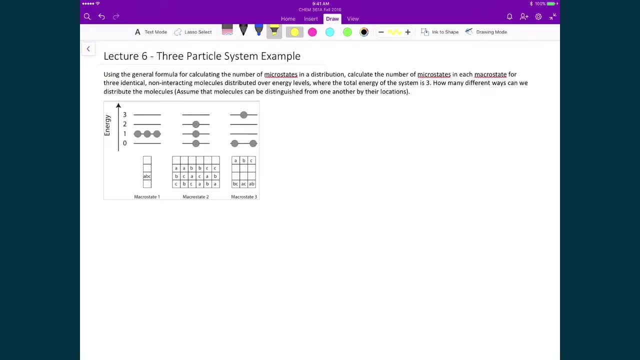 what we're trying to do is just have three identical non-interacting molecules distributed over energy levels where the total energy is equal to 3. And so what we're trying to do is again just determine how many microstates exist in each of the three macrostates, And 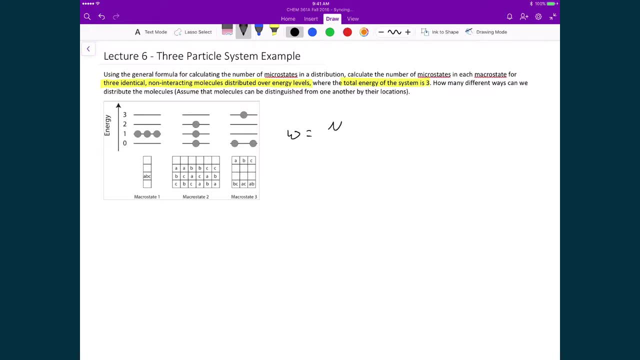 so the way that we calculate this, as was shown on the previous slide, was that we would then take n factorial divided by the product over i of ni factorial, And so in this case, since we've got three particles in our system, that means on top we're going. 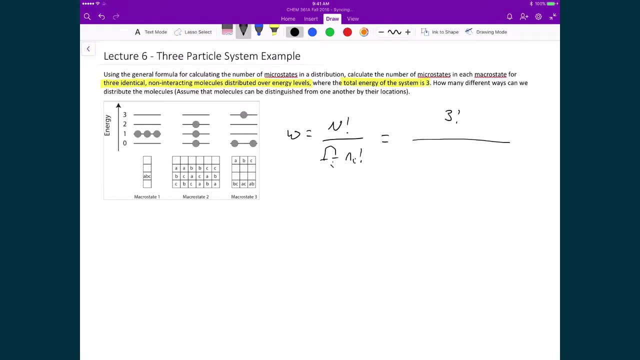 to have 3 factorial, And on the bottom, well, this pi, this capital pi sign, just means the product of what follows, And i basically is going to be equal to 0,, 1, and pi, And 1,, 2, and 3.. So that means, on the bottom, what we're going to have is the number of 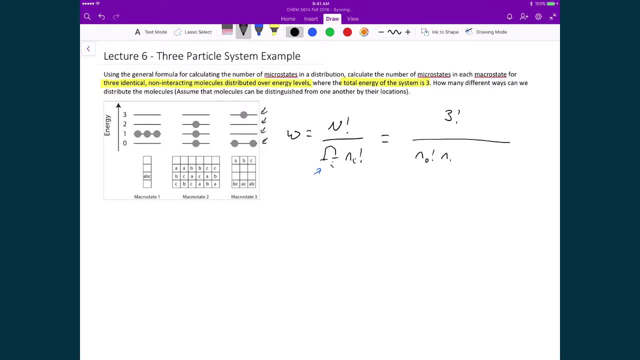 particles in the zeroth energy level factorial times the number in the first energy level factorial times the number in the second energy level factorial times the number in the third energy level factorial. And so we're going to use this general expression then, based on the original definition, to determine how many microstates exist in each of the three. 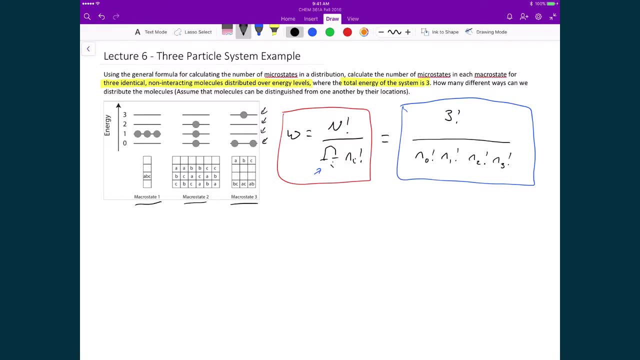 macrostates. Let's now apply this to each of the macrostates. So for macrostate number 1, we have, starting with the general definition, we have n factorial divided by the product over i of ni factorial For this system and, like for the other three, we've got 3 factorial on top And on the 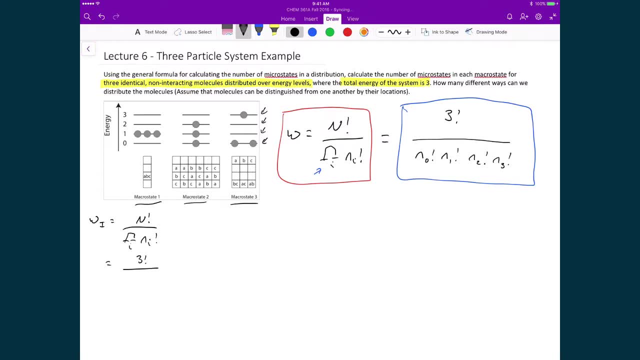 bottom. we're basically again taking the product of the number of particles sitting in each of the energy levels. So n0, there are 0 particles in each of the energy levels, And 1, there are 3. And 2, there are 0. And then 3, there are 0. So that means I'm going 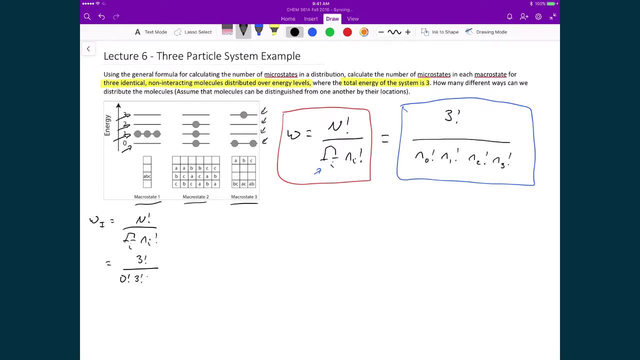 to write: 0 factorial, 3 factorial, 0 factorial, 0 factorial. Now we know that each of these 0 factorials, they're just equal to 1.. And so what we're left with is 3 factorial divided by 3 factorial, which means that there is only one microstate in macrostate 1, which 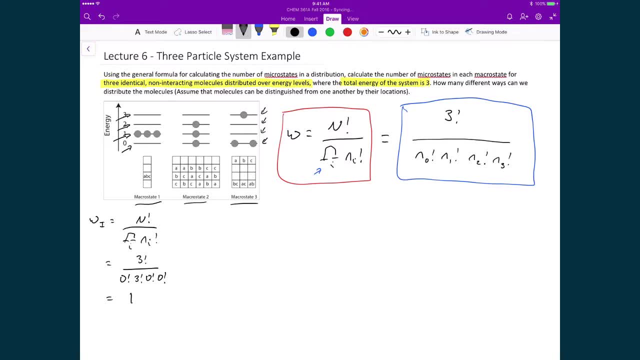 is an answer that we already showed to ourselves And we can see in the image. Moving on to macrostate number 2, we again, we can start with the general definition: n factorial, with the product over i of ni factorial. Well, in this case we still have. 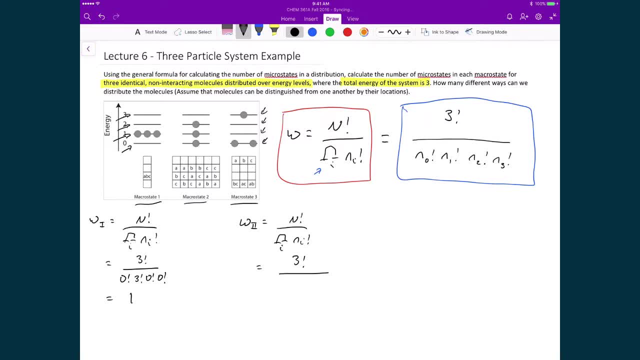 3 factorial. on top, The number of molecules haven't changed. On the bottom, well, we have 1 particle in n0,, 1 particle in n1,, 1 particle in n2, and 0 particles in n3. So that means 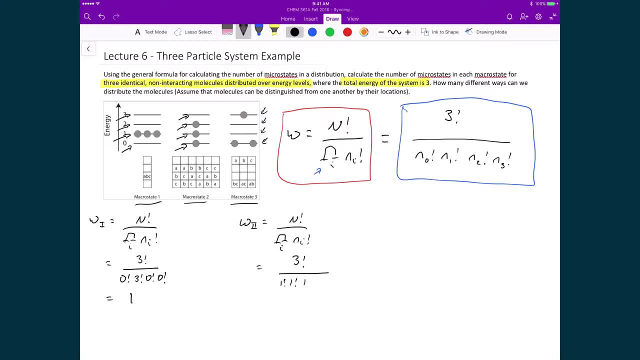 we have 1 factorial times 1 factorial times 1 factorial times 0 factorial And that this denominator is 1 times 1 times 1 times 1.. So it's just 1.. That means we're left with 3 factorial on top, 3 times 2 times 1 over 1, which means that we have a total of 6 microstates. 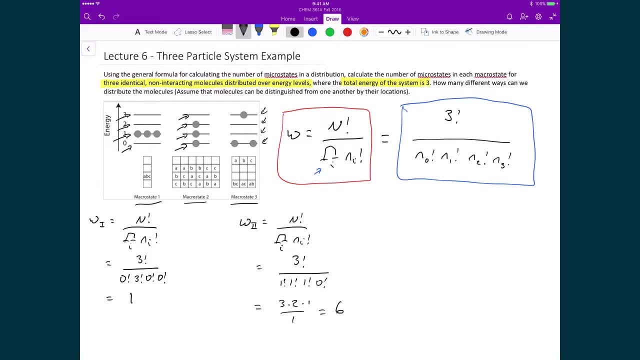 in macrostate 2.. Let's now determine the number of microstates in macrostate number 3.. Here again, n factorial divided by the product over i of ni factorial. What that gives me? again 3 factorial on top. Well, here we have 2 in n0,, 0 in n1,, 0 in n2, and 1 in n3. So we have 2 factorial. 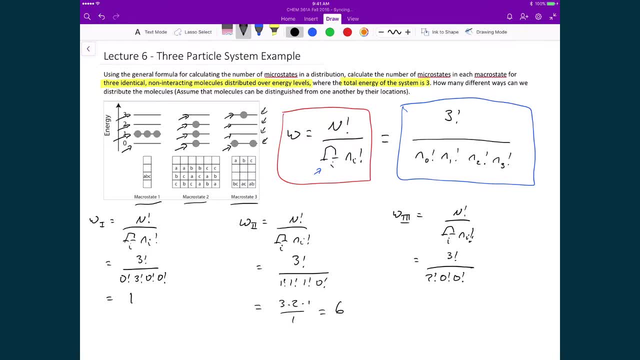 times 0 factorial times: 0 factorial times: 1 factorial. And so in this case, again, the 0s and the 1 factorials. they're just equal to 1. And so what we're left with is 3 times. 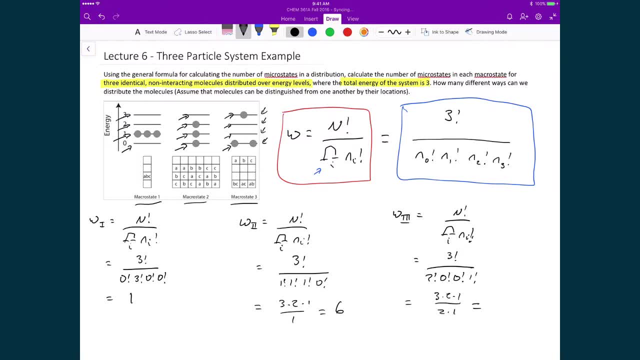 2 times 1 factorial, And so in the end, what we have is 3 microstates in macrostate number 3.. Now, one point I'd like to stress again is this fact that each microstate is equally probable of occurring. 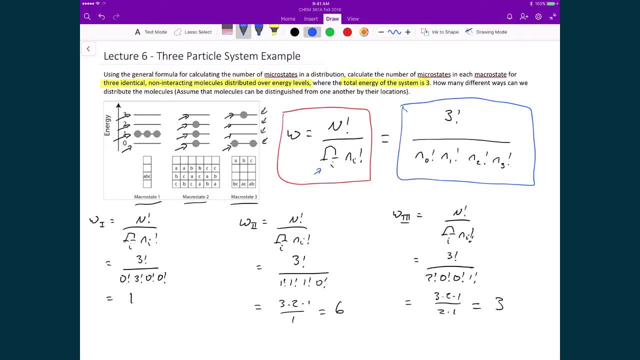 And so that means that we have, over the sum of all of these different microstates, we have 10 in total, And so if each of these, then, are equally likely, then we're left with 1.. Then the one or the macrostate that has the most number of microstates is going to be: 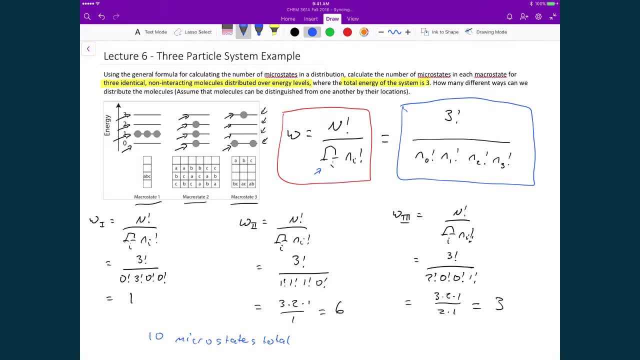 the one that we're going to observe the most. It's the one that's most likely, And so that means, then, that in this case, given this specific system, macrostate number 2 is going to be the one that we're going to see the most, or that we're going to measure the most, because 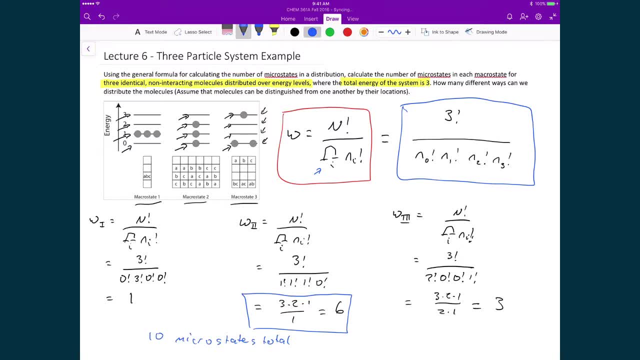 it has 6 microstates, Or in other words, it has the most microstates out of all 3.. And then, in this case, micro or macrostate number 1 is the one we will least see, since there's only one microstate that makes up this one state. What this says to us also is that if 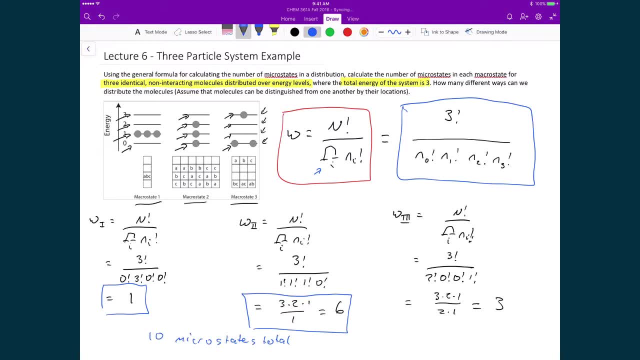 we ended up in macrostate number 1,. if we somehow found ourselves in that state, we would tend to then move towards macrostate number 2, since it is more likely that we would find it, Or there's 6 possibilities out of 10 as opposed to 1 possibility out of 10.. 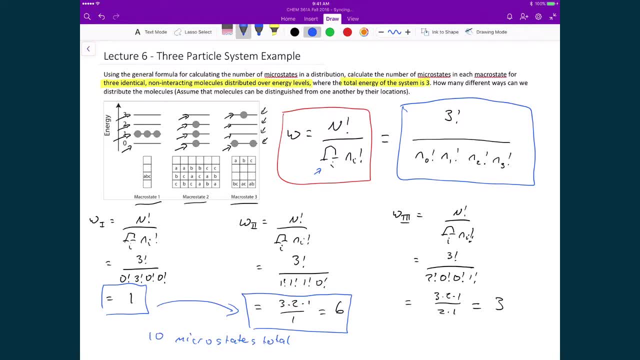 That is, if the system matures or changes into something else, that it would then tend to change into macrostate number 2.. Similarly, if we found ourselves in macrostate number 3, again, we would tend to move towards macrostate number 2 when the system changes simply. 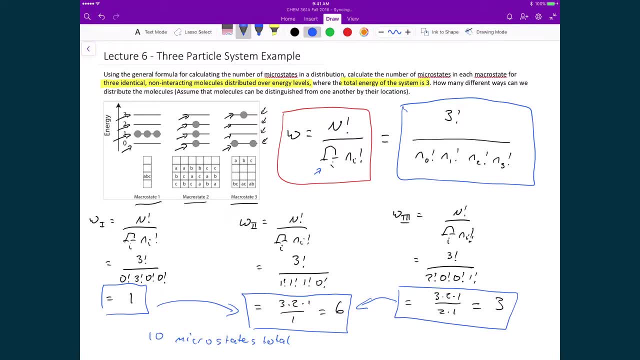 because it is just more likely that we would end up in macrostate number 2, because there's just more possibilities for macrostate number 2 to occur. 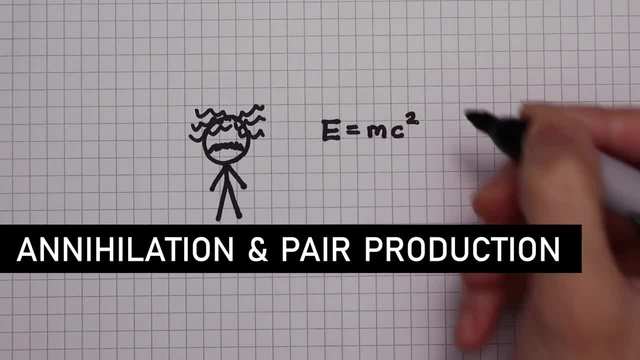 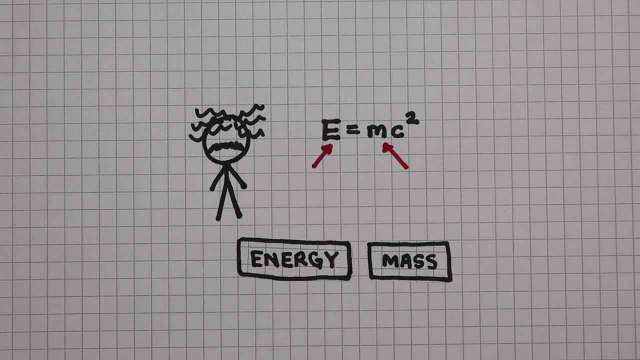 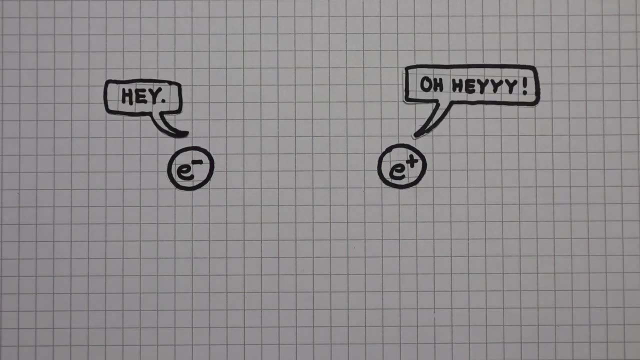 E equals mc squared. Einstein's famous equation tells us that energy and mass are basically manifestations of each other. Energy can be converted into mass and mass can be converted into energy. We witness this in particle physics When a subatomic particle like an electron, 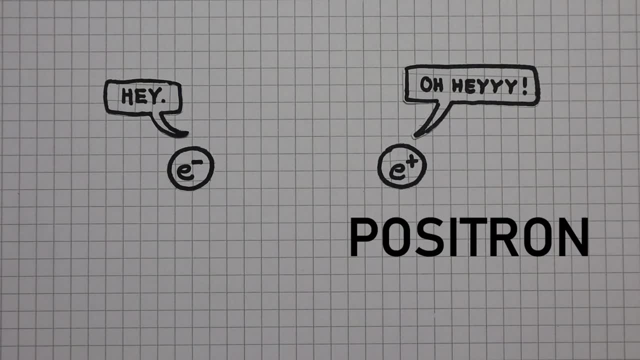 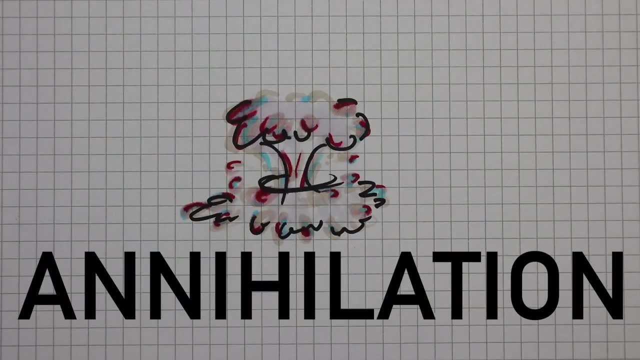 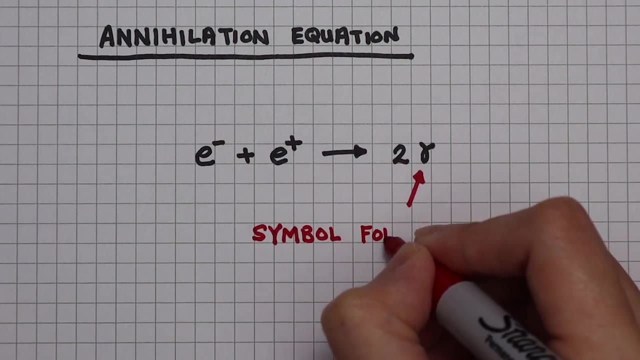 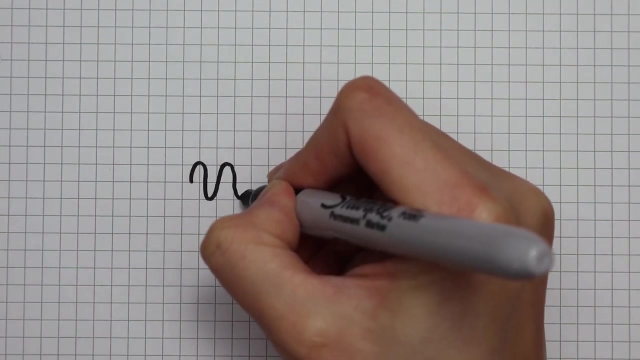 meets its anti-particle, a positron, they annihilate to convert their mass into pure energy. Their energy is carried away by a pair of photons. And now let's have a look at the reverse of Einstein's equation: Energy carried by a photon can be converted into an electron and a positron. This is known as pair. 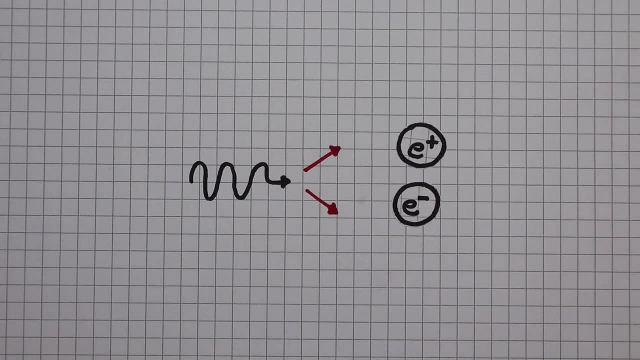 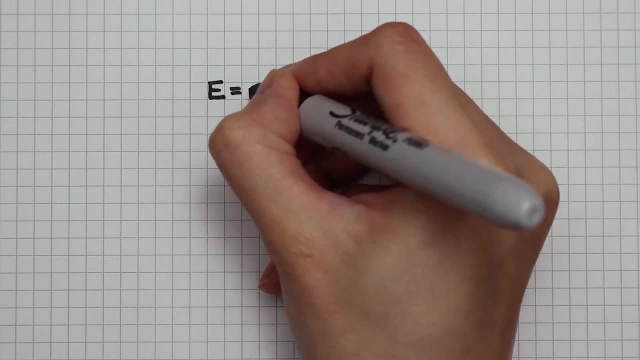 production And on a lucky day, particle physicists might even see them orbits around each other. How much energy does a photon need in order to create an electron-positron pair? The mass of an electron is 9.1 times 10 to the. 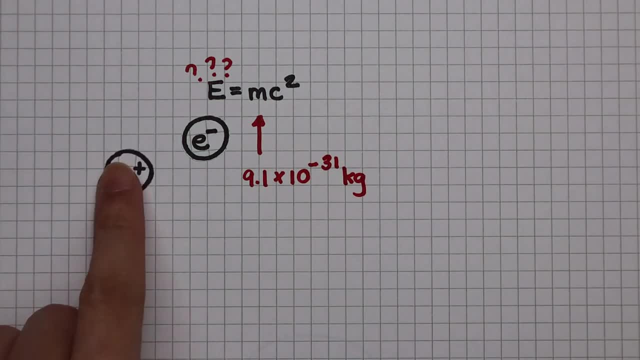 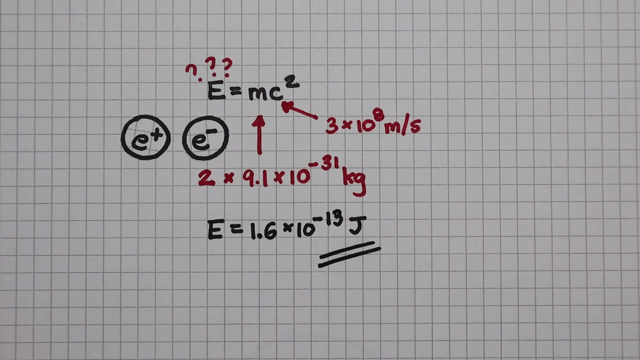 minus 31 kilograms. Since we have an electron and a positron, we need to multiply by two. Speed of light is 3 times 10 to the power of 8 meters per second. So this is the amount of energy a photon needs in order for pair production to happen. Take a guess: which wave in the EM? spectrum carries this much energy, Let us know in the comments below. Thank you for watching. If you enjoyed this video, please like share and subscribe to our channel. See you in the next video. Bye. Thank you for watching. If you enjoyed this video, please like, share and subscribe to our channel.